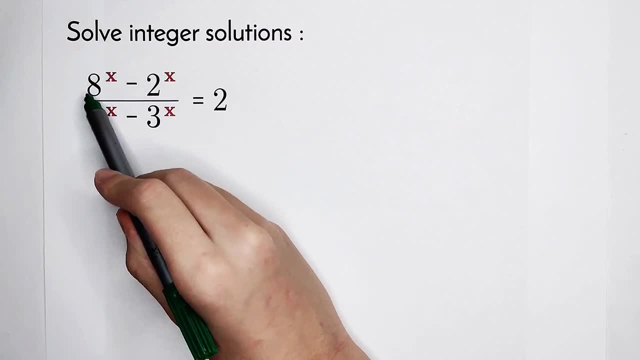 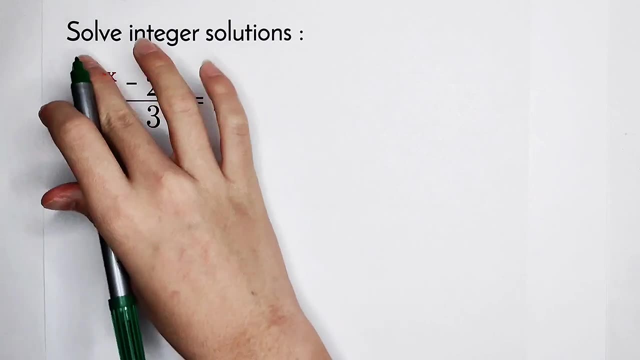 As our first step, we should regard this 8 as 2 to the power of 3,, and this 6 is 2 times 3.. 2 to the power of 3, or 2 to the power of x is equal to 2 to the power of x, then, or 2 to the power of 3.. 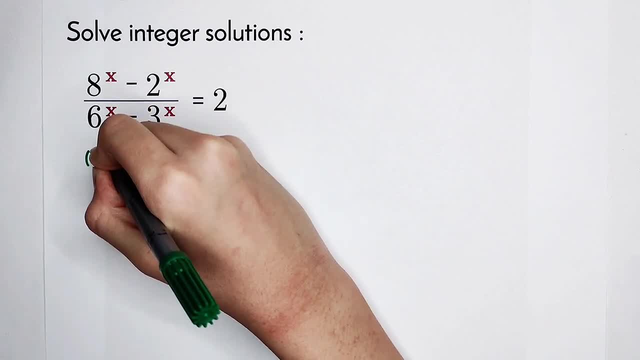 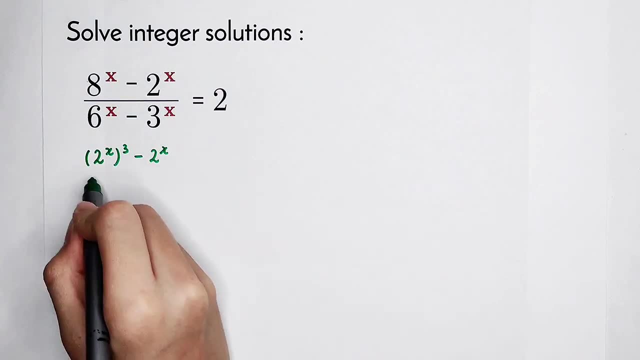 So it is 2 to the power of x, then, or 2 to the power of 3, minus 2 to the power of x. Now here comes the denominator. Since 6 is 2 times 3, then 6 to the power of x is 2 times 3,, then, or 2 to the power of x. 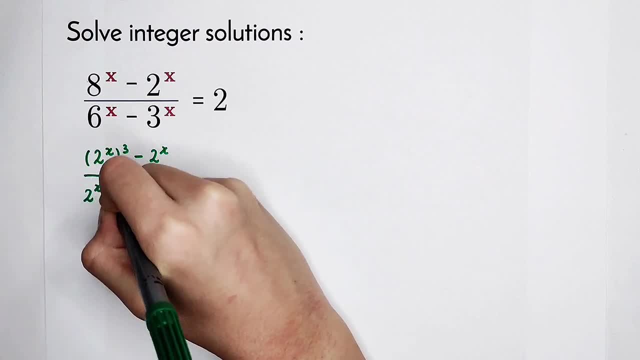 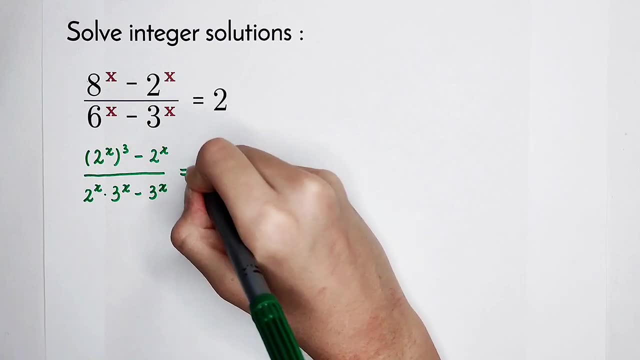 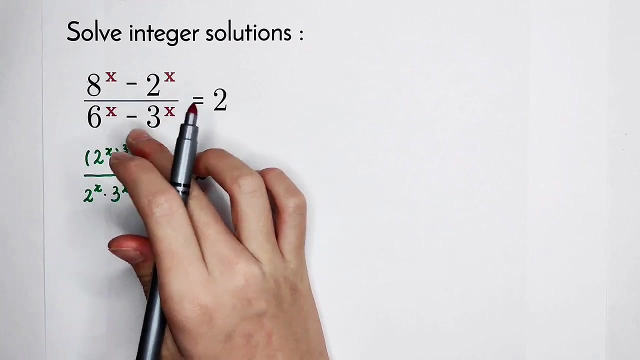 It is equal to 2 to the power of x times 3 to the power of x, then minus 3 to the power of x, And then is equal to 2.. Now, what should we do? The numerator 2 to the power of x, or cube, then minus 2 to the power of x. 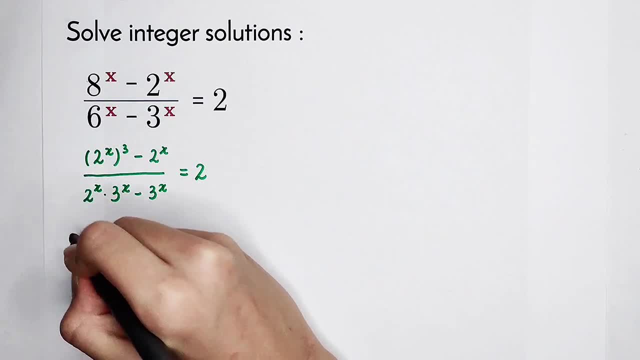 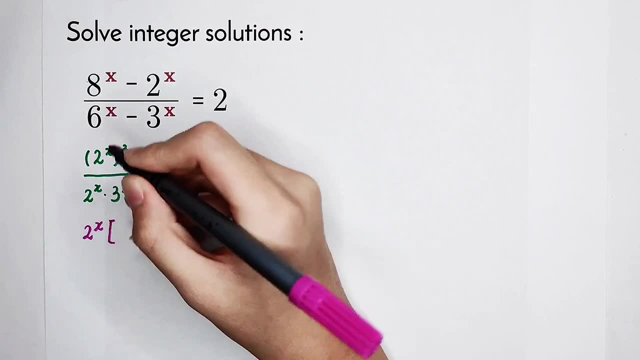 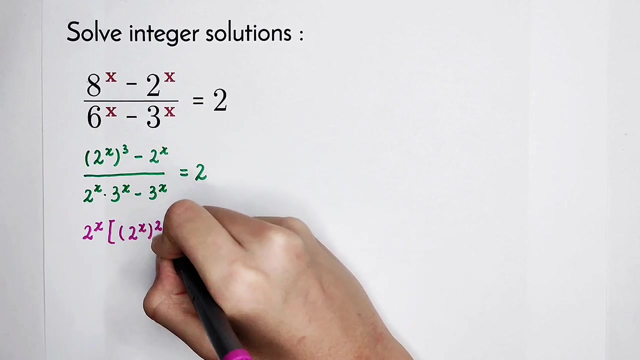 We can take out a 2 to the power of x, So it is 2 to the power of x. and then what's in the bracket? It is 2 to the power of x and then, or squared And then minus. 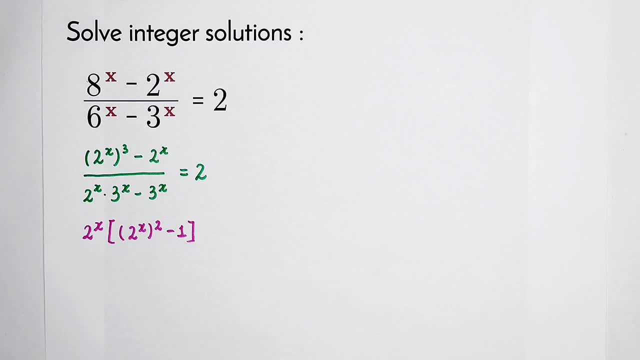 Minus 1.. Nice, Now I'm going to multiply by this denominator on the both ends sides, Then it is equal to 2 times this In this term. I can take out 3 to the power of x, And then what's in the bracket? 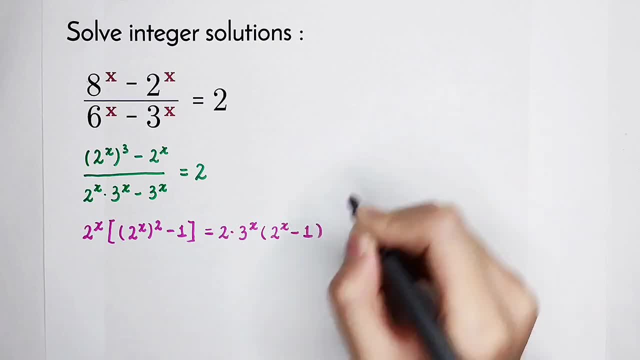 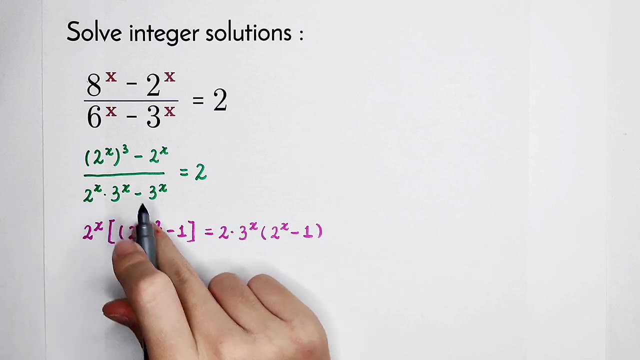 2 to the power of x minus 1.. Good, For our next step, I'm going to use a formula: A A squared, then minus b, squared is equal to a plus b, then times a minus b. So this: 2 to the power of x, then, or squared, then minus 1.. 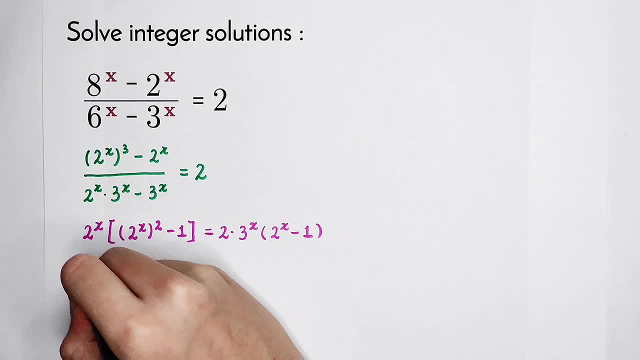 This one. I can regard it as 1 squared, So it is 2 to the power of x, then times. a is 2 to the power of x, b is 1.. First add them together and then times. 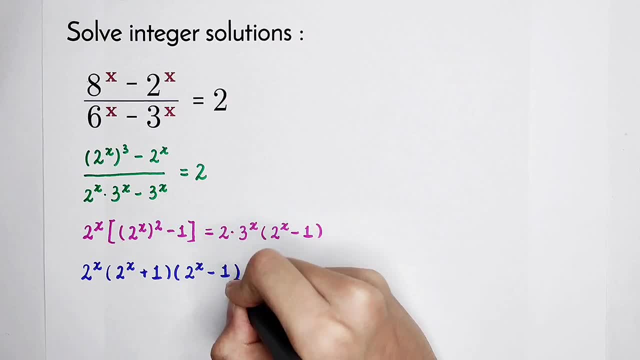 The subtraction, The third binomial formula: 2 times 3 to the power of x and then times 2 to the power of x minus 1.. All of you must have noticed: 2 to the power of x minus 1.. 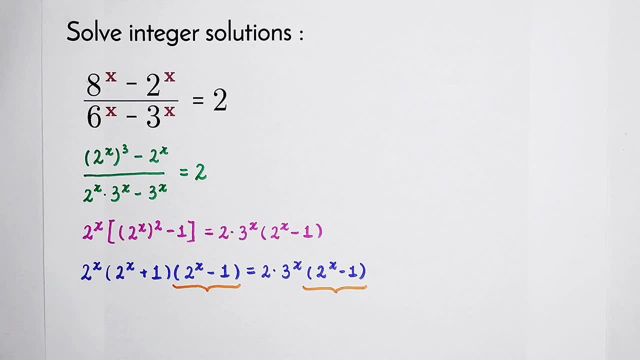 Cancel. No, no, no. The only way is it is not equal to 0. But can it be 0?? 2 to the power of x, then minus 1 is 0, that means 2 to the power of x is equal to 1.. 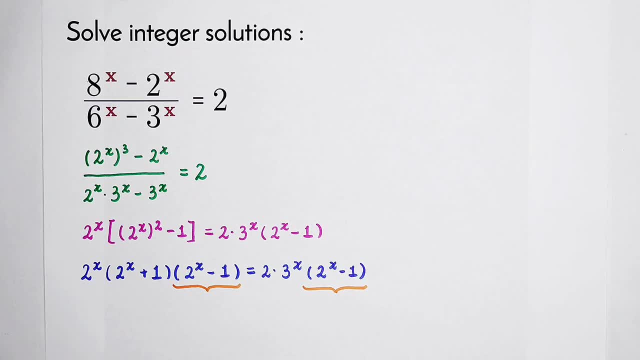 Can 2 to the power of x is equal to 1?? Of course it can when x is equal to 0.. But can x be 0?? No, Because when x is equal to 0, it can be 0.. 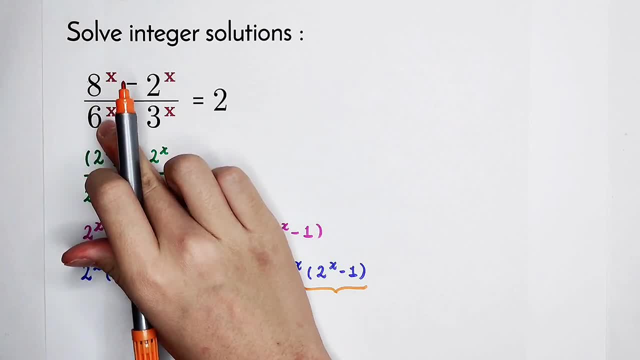 No, Because when x is equal to 0,, it can be 0.. Because when x is equal to 0, it can be 0.. 6 to the power of x minus 3 to the power of x is the denominator. 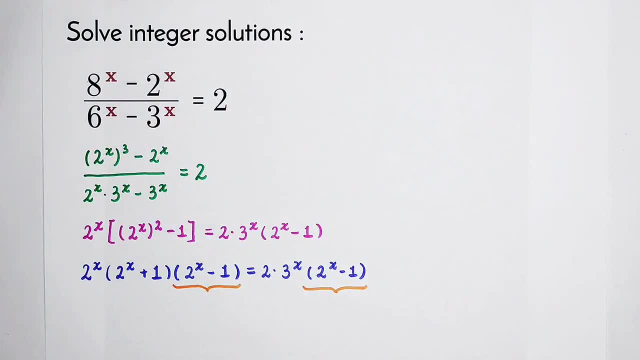 Then it will be 1, minus 1 is 0. But the denominator can never be 0. So x can not be 0. That means x can never be 0. So that means we can cancel this 2 to the power of x minus 1, on the boson signs. 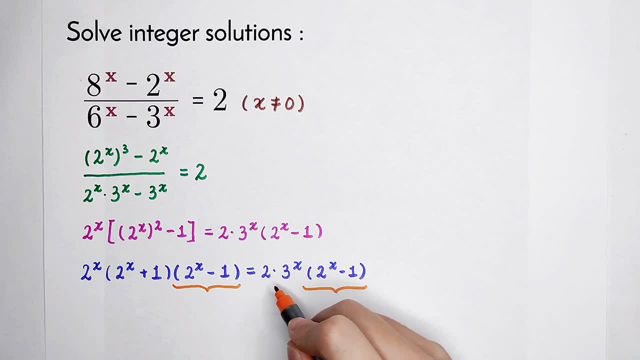 For the next step, we can divide it by 2 on the both hand sides. Then this 2 to the power of x will be 2 to the power of x minus 1.. 2 to the power of x minus 1.. 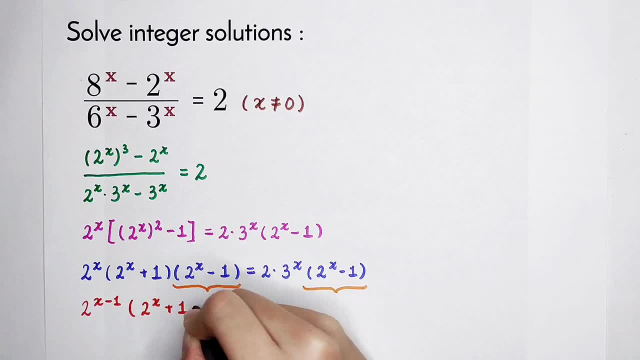 And then times 2 to the power of x plus 1.. 2 divided by 2, it will be 1.. So ignore 3 to the power of x. This guy looks not so nice, But maybe you have found- when x is equal to 1, you can get that 1 times 3 is equal to 3.. 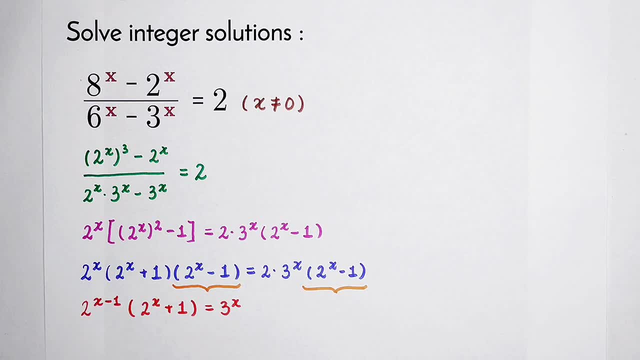 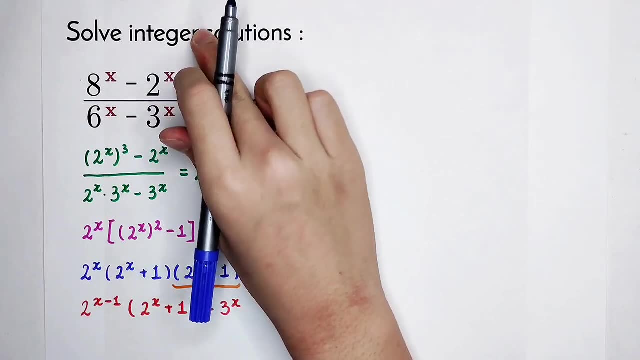 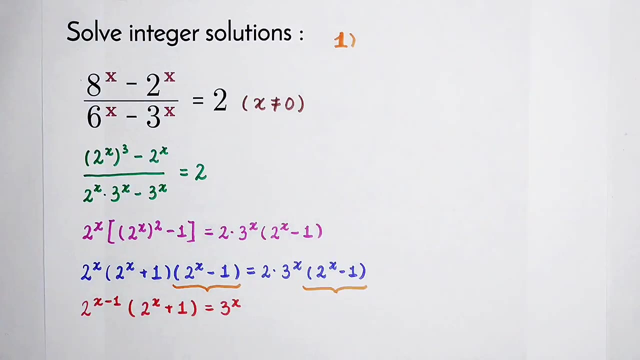 The equation can be hold. But now we have to find all of the integer solutions of this equation. Pay attention, it is integer, not positive integer. The first thing: x is equal to 1.. When x is equal to 1, this equation can be hold. 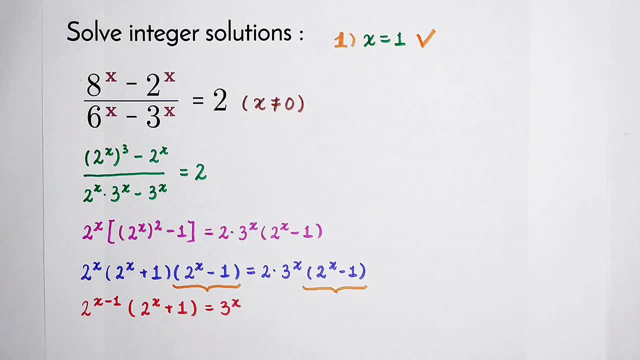 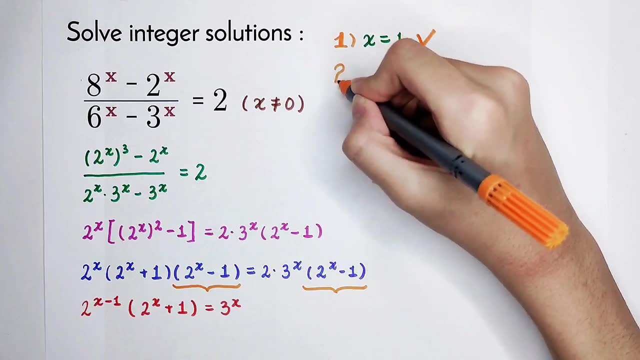 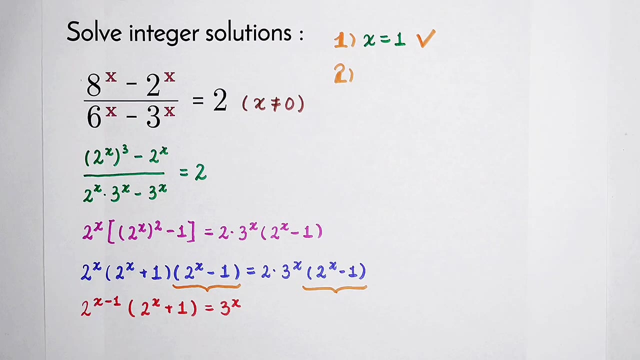 8 minus 2 is equal to 6.. 6 divided by 3 is equal to 2.. It is correct And we have our second case, The second case when x is not equal to 1.. Of course, It also cannot be 0.. 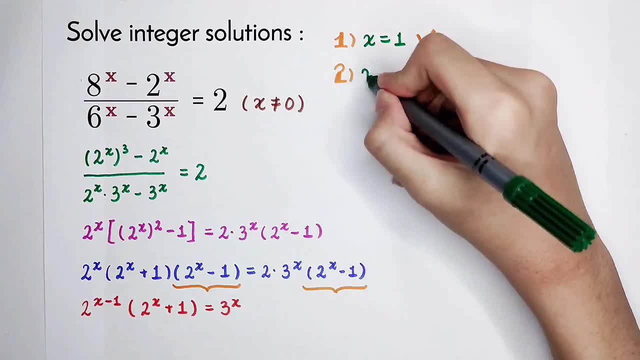 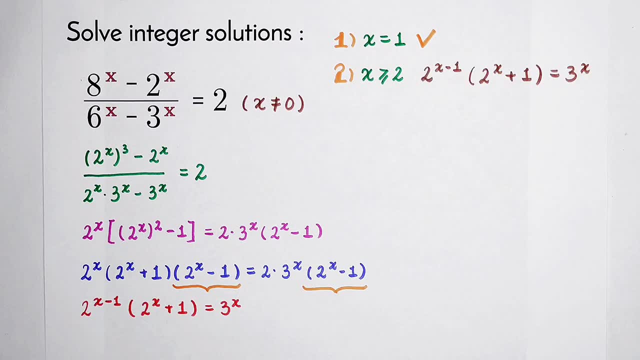 Now we can explain. x is greater than or equal to 2.. And x is an integer, Since x minus 1 and x are always positive integers. So now we have to pay attention to their parities. The base is 2.. 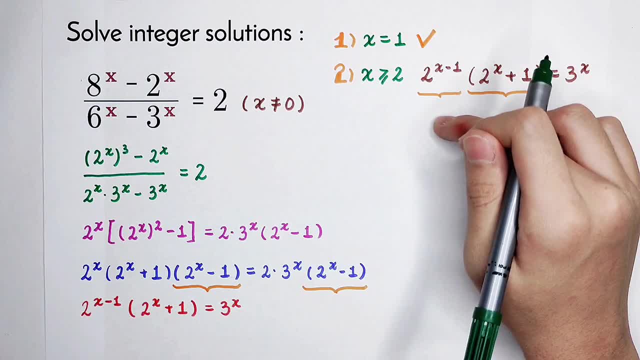 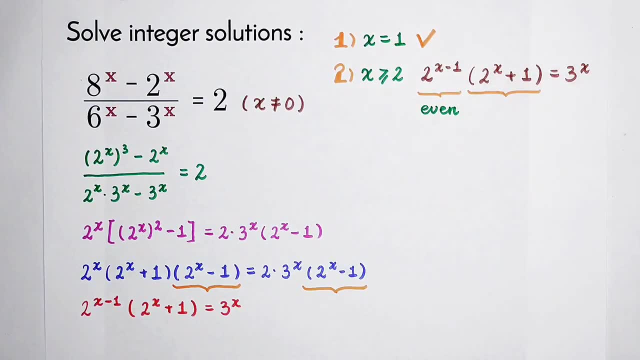 2 to the power of any positive integers, the results are always even. 2 to the power of any positive integers, then plus 1, are always odd. And 3 to the power of x, the results are always odd. But 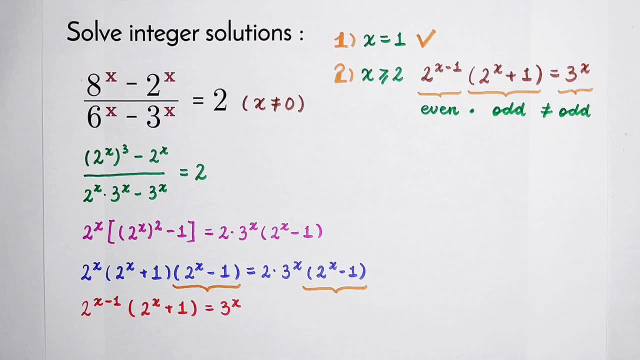 An even number, Then times an even number Is even Cannot be odd. Of course We also have the third case. The third case is when x is negative. Now substitute x is equal to negative n into this equation. a to the power of negative x is equal to 1 over a to the power of x. 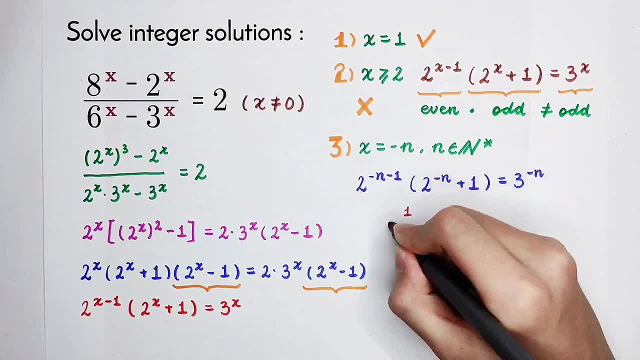 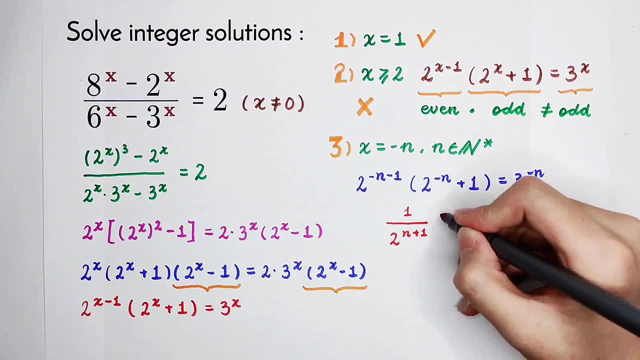 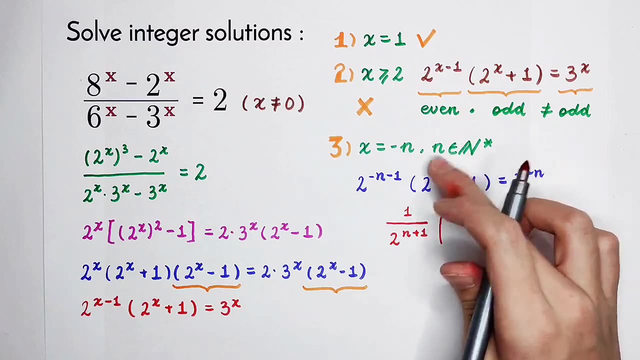 So now It is 1 divided by 2 to the power of n plus 1.. And then times 2 to the power of negative n, then plus 1.. This 2 to the power of negative n is equal to 1 divided by 2 to the power of n.